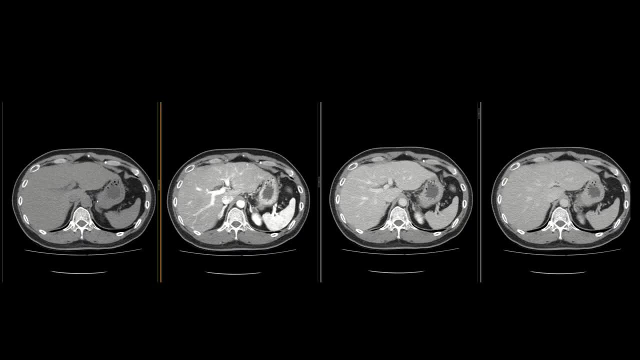 liver lesions in a further video. So to start, let's look at this four-phase scan of a normal liver. You'll notice that the appearance and attenuation of the normal liver depends heavily on the phase of IV contrast. but the normal liver is pretty homogeneous on all of these phases. 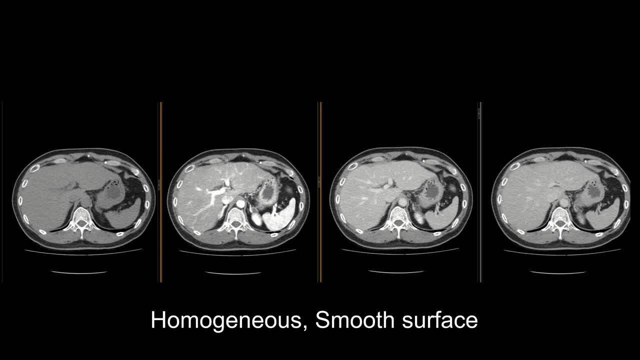 As you know, normal liver has a dual blood supply: about 75% from the portal venous system and about 25% from the hepatic artery. Here are the four phases we're looking at here. So we have one on the left, a non-cortical. 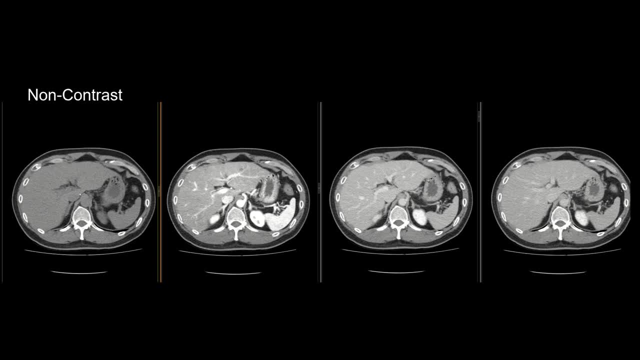 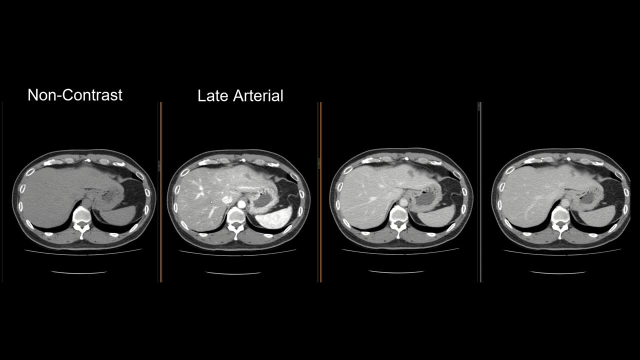 Contrast acquisition before IV contrast was given. Two: we have a late arterial phase acquisition around 35 seconds after injection, with the arteries opacified, the portal vein opacified, but not yet the hepatic veins, as you can see here. Notice that the background liver 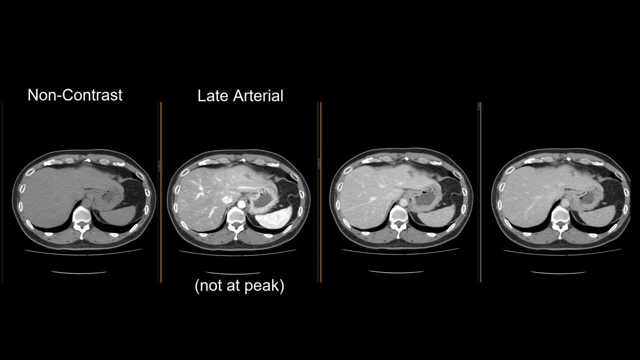 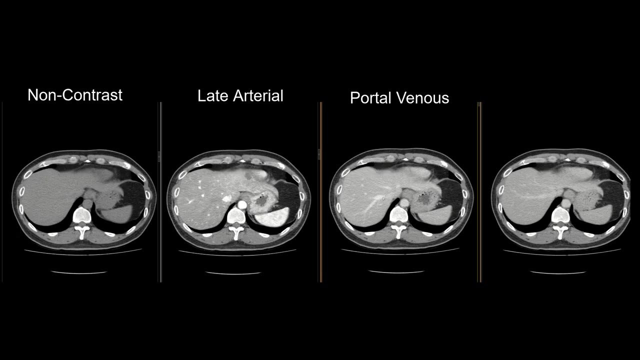 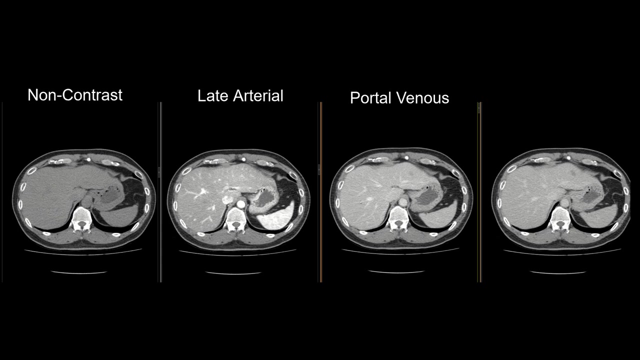 doesn't enhance that much. Remember, most of the supply is portal venous. Three: we have a portal venous phase acquisition around 75 seconds after injection, with the hepatic veins, as you can see, now opacified And the background liver is also now closer to peak enhancement. So background 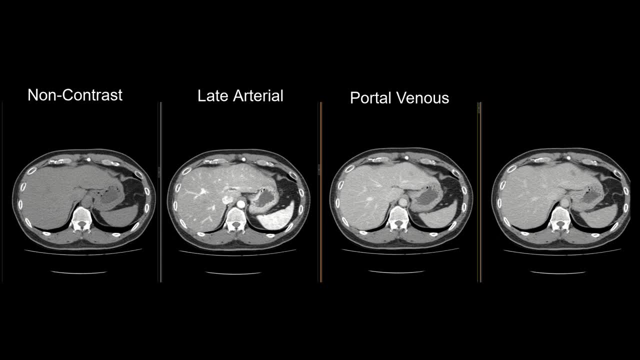 liver is pretty bright. And then four: we have a more delayed phase here on the right or equilibrium phase. This one was acquired at about a few minutes after injection, With contrast now moving out of the liver and the attenuation of background liver now less than it was on portal. 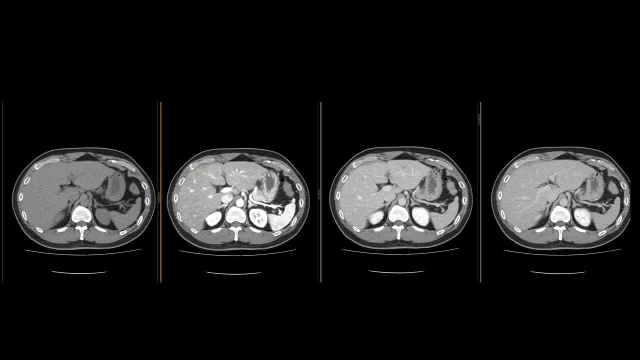 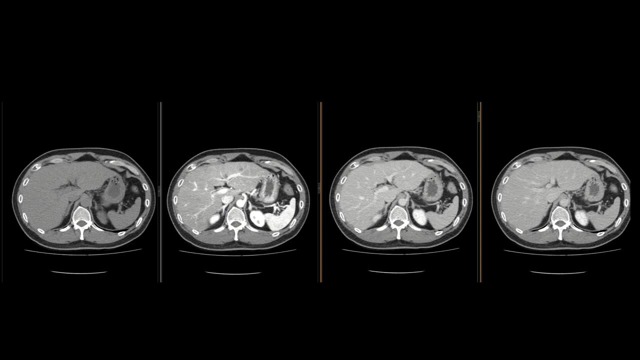 venous phase. In routine imaging of the entire abdomen and pelvis we most commonly image in portal venous phase, So we most commonly see the liver in portal venous phase. We also- not uncommonly- will image without contrast, So you'll see the liver on non-contrast- only a bunch as well. So we're going to 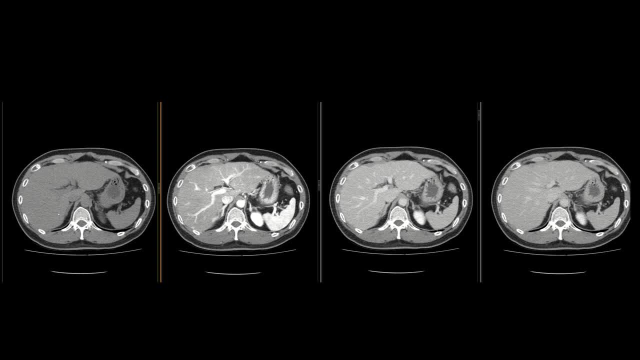 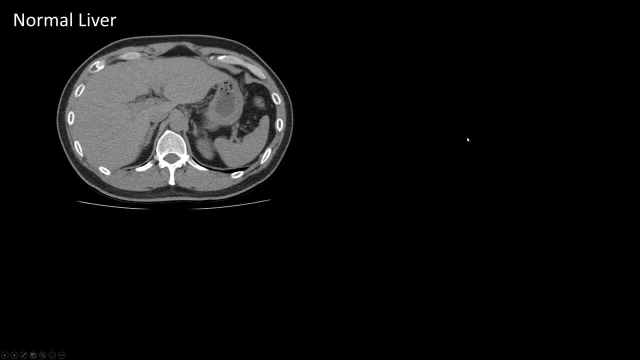 see the liver on non-contrast only a bunch as well, And then usually for dedicated liver evaluation, like if we're characterizing liver lesions, for example, we're going to see all of these phases together on the same examination. All right, so let's cut to the chase. When you're looking at the 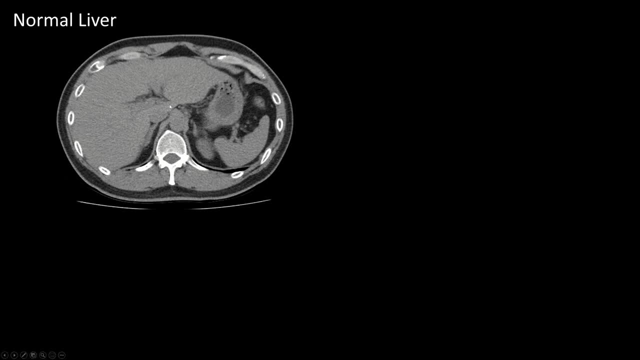 background liver on CT, the two most common abnormalities that you will see in clinical practice are fatty liver disease, aka diffuse hepatic steatosis- and cirrhosis. These are also things that you want to accurately diagnose, so we're going to spend most of our time on these. This is a normal liver, on non-contrast. 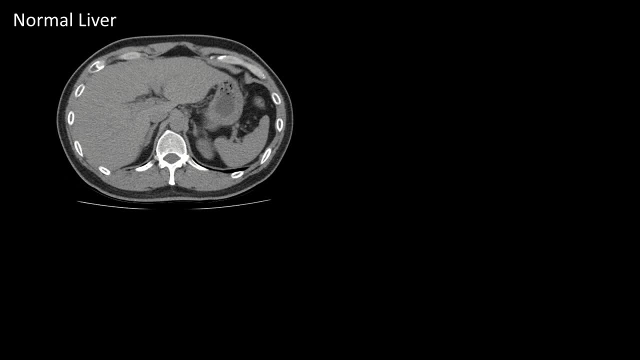 acquisition. Background: liver has a normal attenuation, most commonly in the 55 to 65 ounce per unit range. Here it's about 55 ounce per units. Remember that fat has a lower attenuation than water and soft tissue Fat is darker, So diffuse fatty infiltration in the liver is going to reduce the. 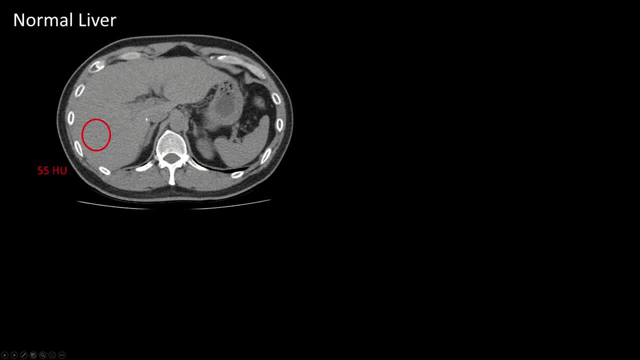 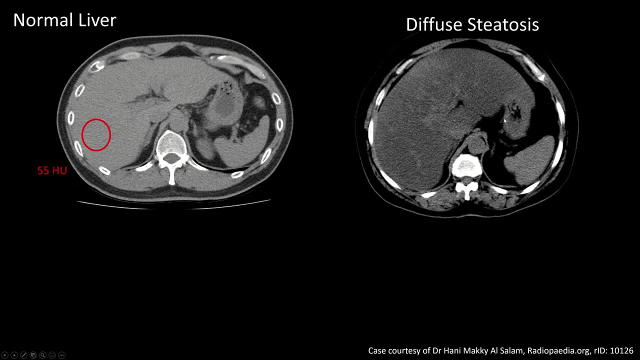 attenuation of background liver or make it look darker. So here is a very fatty liver on non-contrast acquisition with a much lower attenuation of the liver, about 25 ounce per units, in this case On CT. the non-contrast acquisition is actually the best for looking for fatty liver, Once you give. 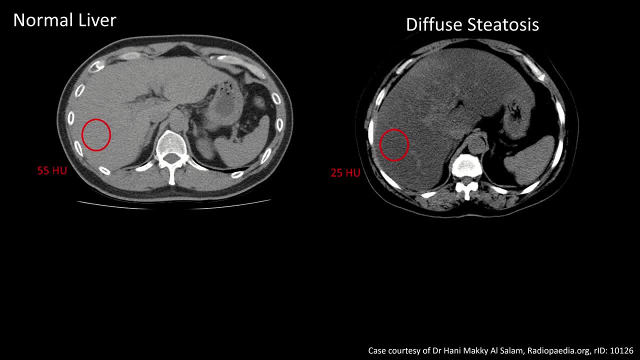 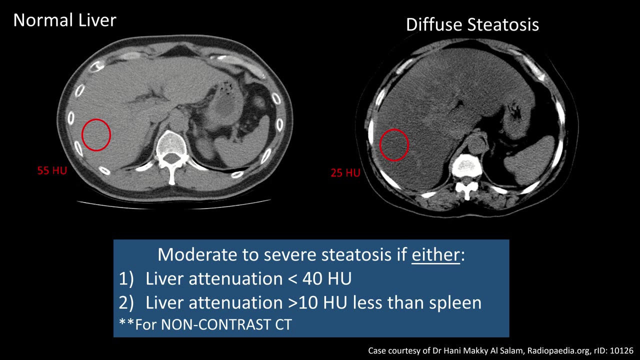 the patient IV contrast, which is bright, remember contrast. timing really affects the attenuation of the liver, so it gets a little bit tougher to know if there's fatty liver or not. On a non-contrast CT we can confidently say that there is fatty liver if either of the following are true. One: 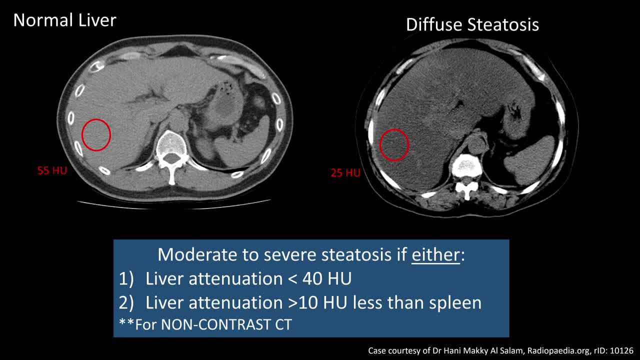 the background liver attenuation is less than 40 ounce per units, as it is here, And two if the liver attenuation is more than 10 ounce per units less than the attenuation of the spleen, as it is here as well. Now, these rules are good for moderate to severe steatosis. CT is actually not that sensitive for picking up patients with more mild fatty liver. 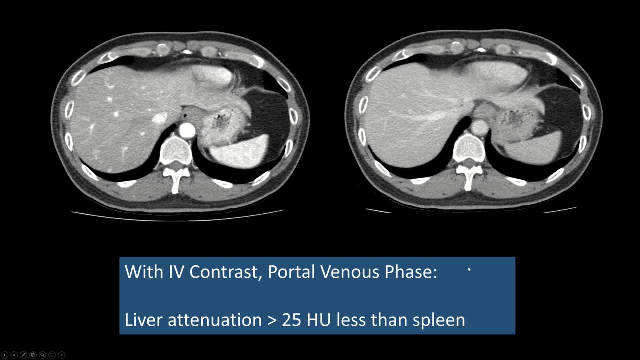 So, as I mentioned, once you give IV contrast it's a lot harder to know if there is fatty liver or not. But a pretty reliable criteria on portal venous phase is the liver attenuation being more than 25 ounce per units, less than the spleen attenuation. 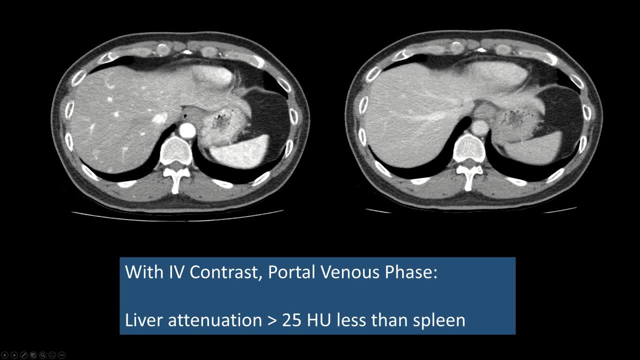 So here are some post contrast images, let's say, in two patients and we have some ROIs that we've drawn here on the liver and the spleen. So let's take a look at the fresh blood sample. We're gonna see a detaillation of heralding and we've found a clear tr. 1957judges. 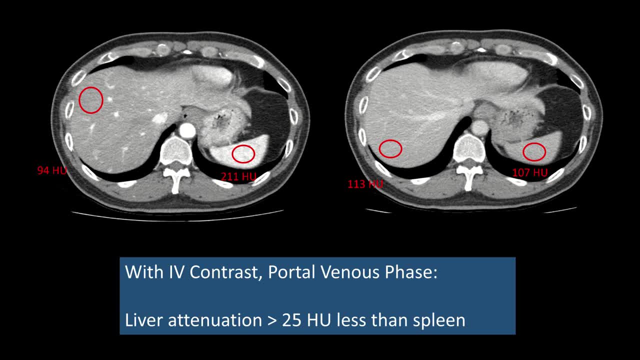 and the spleen in these patients. so what do you think? do these patients have fatty liver or not? so these are both images of a patient with a normal liver that is not fatty, so some of you might have called this first liver fatty, right, the difference between 211 and 94 is much greater than 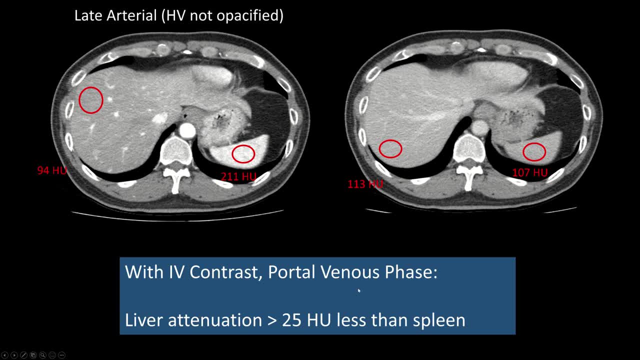 25. so this rule here only applies when it is a portal venous phase. this is a late arterial phase and on this image here on the left you'll notice that the artery is very high attenuation. the portal veins are opacified, but the hepatic veins are not yet opacified. this is a late arterial phase. 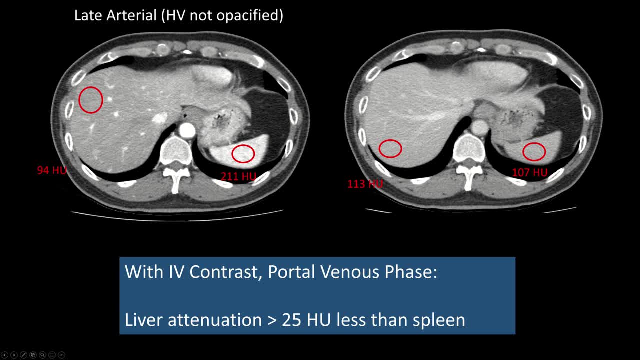 so the background liver, as we know, is going to be pretty dark. the spleen is usually very enhancing or very bright. so you're going to over call for fatty liver if you try to apply this rule in a late arterial phase, calling fatty liver on a late. 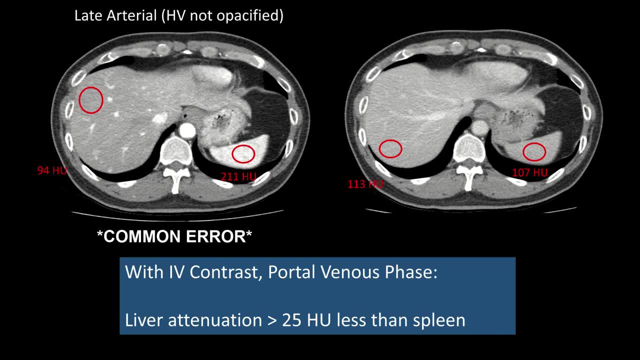 arterial phase acquisition is the most common mistake that I see residents making when they use or try to apply this particular rule. so remember, if it's a post-contrast study and the hepatic veins are not yet opacified, you can't tell if the liver is fatty, unless, of course, it happens. 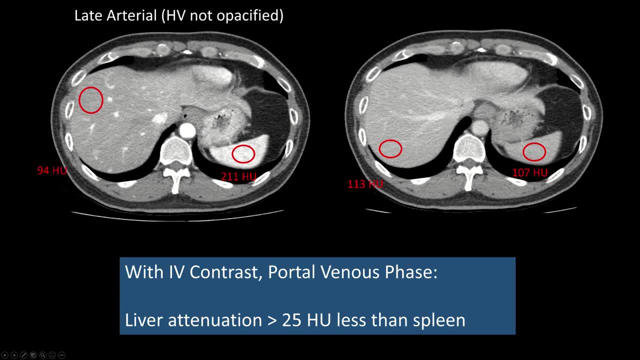 to be under 40 ounce-feelings, which would be pretty rare. this image here on the right is a portal venous phase. notice that the hepatic veins are opacified here and in this case, based on the attenuations of the liver and the spleen, we would not be able to call this liver a fatty liver if you take a few things away from. 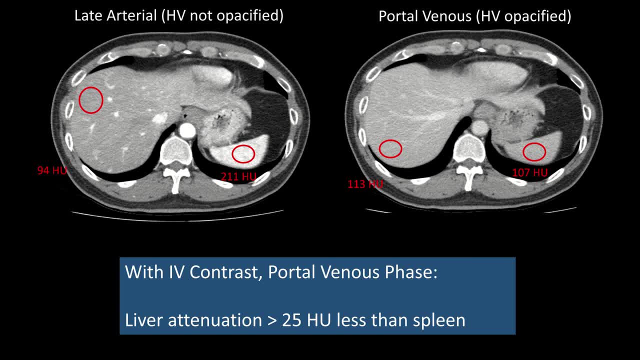 this discussion. remember one: fatty liver is super common and you're going to see it all the time on CT, so you need to know these rules. two: routine CT is not very sensitive for mild hepatic steatosis or mild fatty liver, but it's really good for moderate to severe fatty liver. we can call fatty. 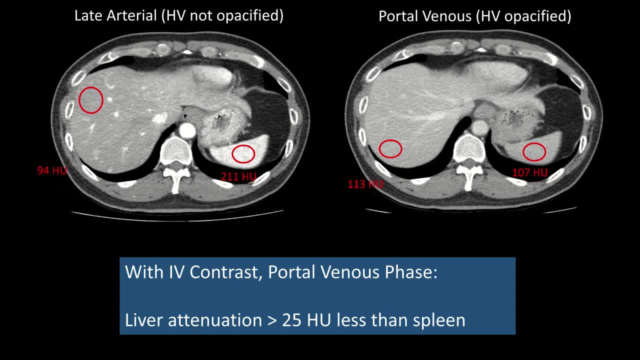 liver confidently on a non-contrast scan when attenuation is less than 40 ounce-feel units or more than 10 ounce units less than the spleen three. once we give contrast, things get a little tougher and less sensitive. but if the liver is more than 25 ounce, 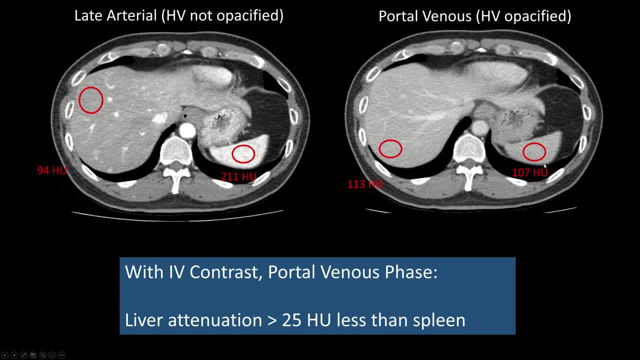 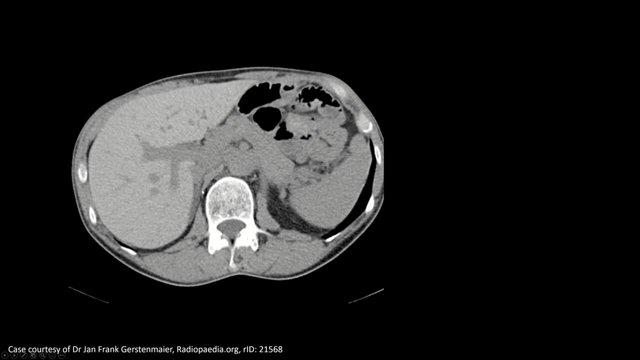 units less than the spleen on portal venous phase. again, only once the hepatic veins are opacified, then we can also call fatty liver. moving on, this is a non-contrast acquisition of the abdomen. we've drawn an ROI here on the liver and the liver. 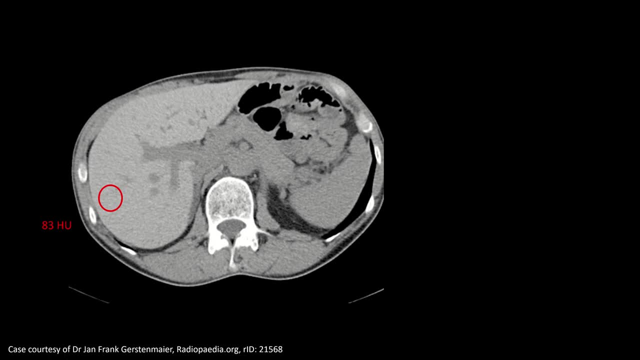 measures 83 ounce-feel units, remember the normal liver is most commonly somewhere between 55 and 65, so the attenuation is pretty high here, the background liver being too high. attenuation is something that you're going to see less frequently than fatty liver and clinical practice, but when 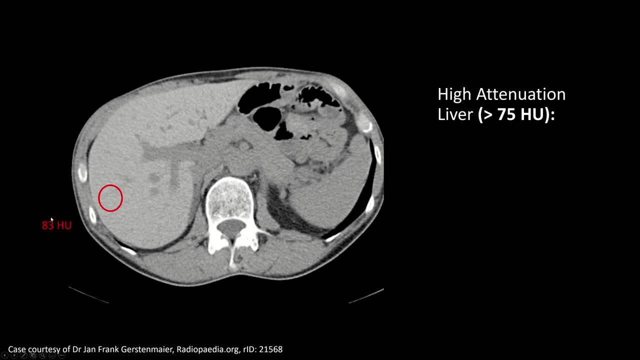 the background: liver measures greater than 75 ounce units on non-contrast acquisition- that's considered abnormal. the most common causes are usually listed as hemochromatosis, hemo siderosis, Wilson's disease, glycogen storage disease, medications like amiodarone gold, etc. but let's 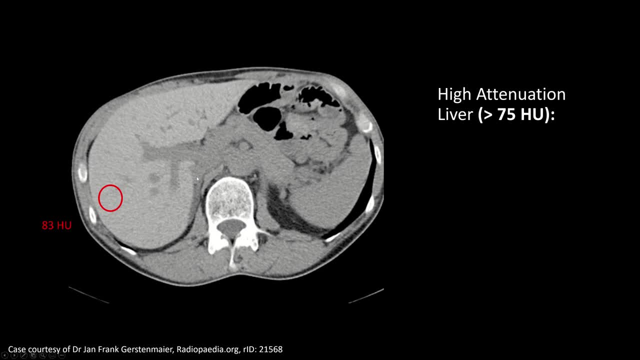 simplify this a little bit. increased attenuation in the liver is most commonly going to be caused by iron deposition and you're going to see iron deposition in the liver in, you know, hemo siderosis or hemochromatosis. that's going to be the most common cause: iron deposition, copper deposition is.